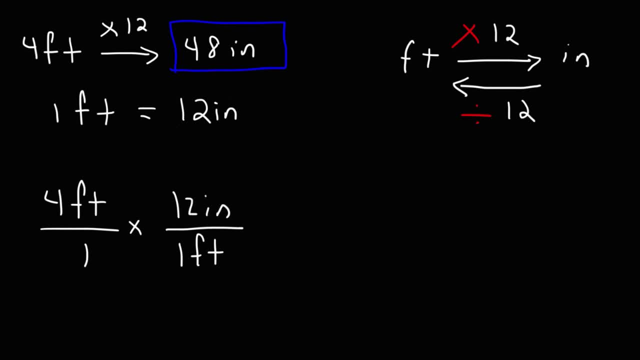 So when we set it up this way, we can see that the unit feet will cancel, And the fact that 12 is on top of the second fraction tells us that we need to multiply those two numbers. So it's four times 12. And that gives us 48 inches. So go ahead and try these two example problems: Convert 8.5 feet into inches And also 2.7 feet. 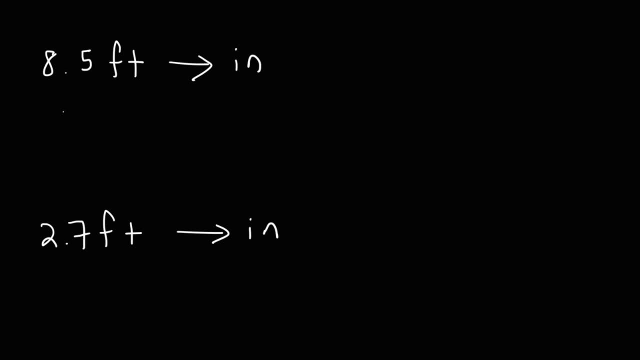 Into inches. So, starting with what we're given, we're going to write 8.5 feet over one, And then we know that there's 12 inches in one foot. So we're going to set it up in such a way that these units cancel And we're going to multiply the numbers on top of the two fractions. So it's 8.5 times 12, which is 102.. 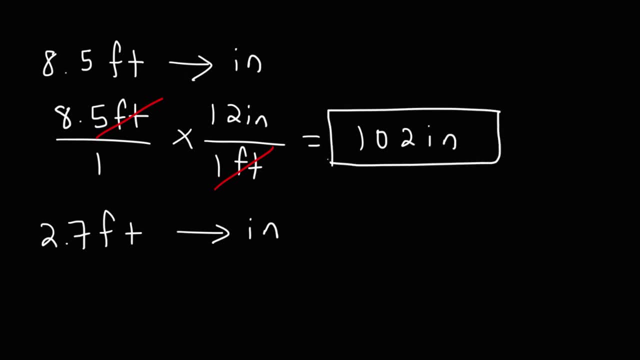 So that's it, And that's it for the first example. And for the second example you just got to follow the same process, So it's going to be 12 inches over one foot in the second fraction, And then we just got to multiply 2.7 by 12.. So 2.7 times 12 is 32.4 inches, And so that's how you can convert from feet into inches. 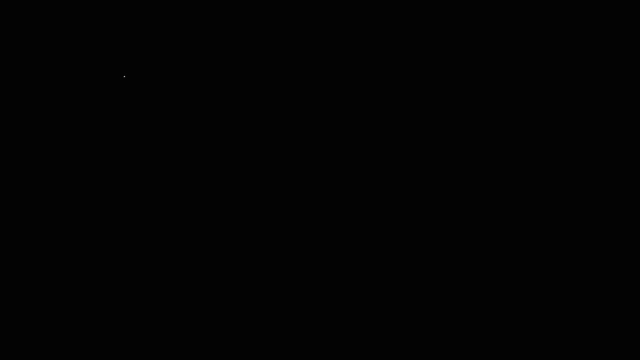 But now let's talk about going the other way, that is, from inches to feet. So let's say we have 36 inches, How can we convert that to feet? So in this case, going from inches to feet, we'll need to divide by 12.. 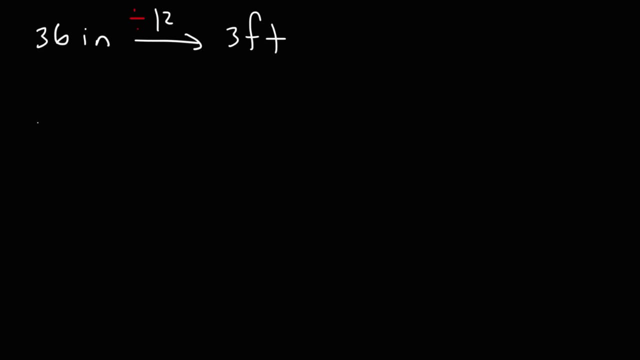 So the answer is going to be three feet. Now to set up the conversion process. we're going to put the unit inches on the bottom, So keep in mind there's 12 inches in a foot, So these units will cancel. And because the number 12 is on the bottom part of the second 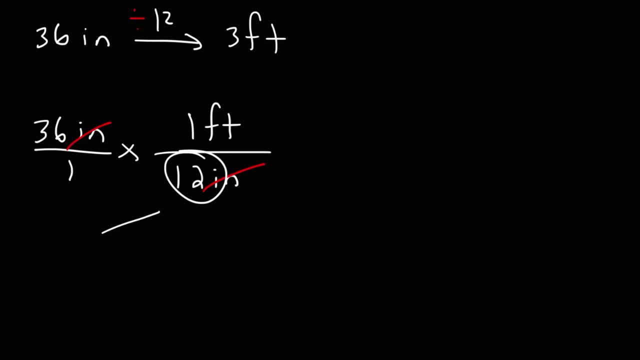 fraction. that tells us that we need to divide 36 by 12.. And so 36 divided by 12 will give us three feet. You could try this one. Convert 52 inches into feet. Feel free to pause the video and try that example problem. So we're going to start with what we have here. 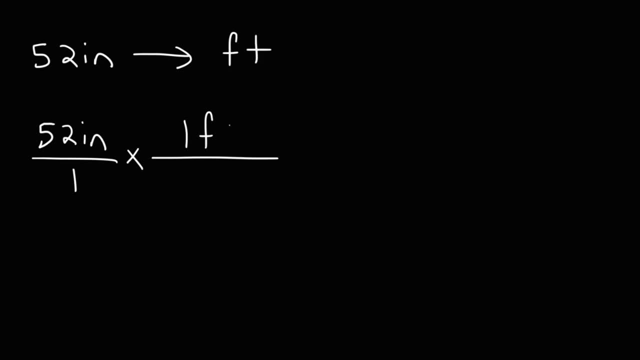 So we have 52 inches, and one foot is equal to 12 inches, So it's going to be 52 divided by 12. And so the answer is going to be 4.33 feet. It's 4.3 repeated, but that's the rounded answer. 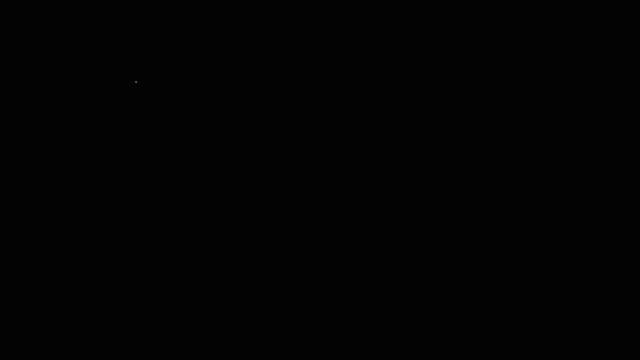 Now here's a challenge question for you: How would you convert 216 squared into feet squared? How would you do that? So, once again, you need to start with what you're given Now. we know that one foot is equal to 12 inches, But notice that the unit is squared. 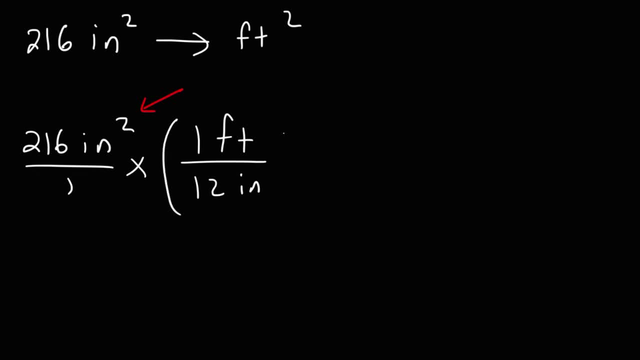 This is not squared, So what we need to do in this case is we need to square the conversion factor. So it's going to be 216.. Divided by 12 squared, 12 squared is 12 times 12, which is 144.. 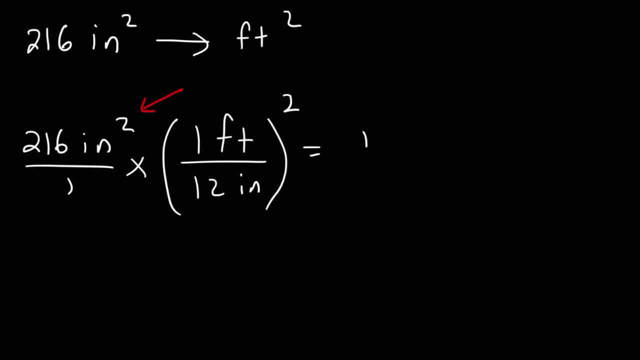 So it's 216 divided by 144.. And that will give you 1.5 square feet. So that's how you can convert from square inches to square feet. So here you're dealing with units of area as opposed to units of length. 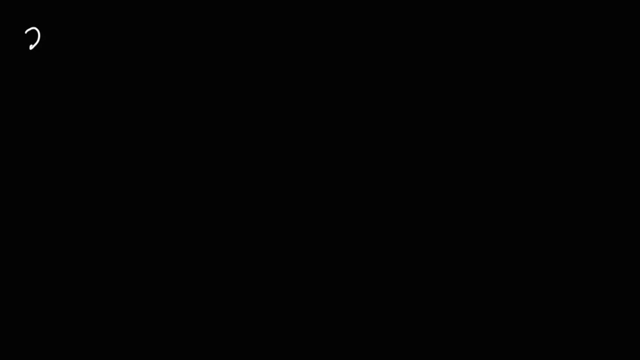 Let's look at another example. How would you convert 2.4 square feet into square inches? Go ahead and try that. So once again, we're going to start with what we have Now. we have square feet on the top of the first fraction. 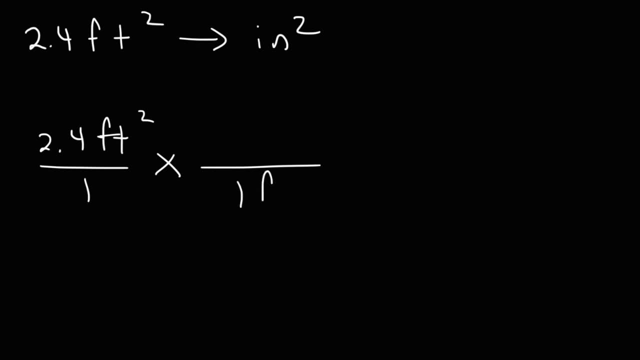 So we need to put the unit's feet on the bottom of the second fraction. One foot is 12 inches, So to get feet squared we need to square the conversion factor. So this time we're going to multiply 2.4 by 12 squared.